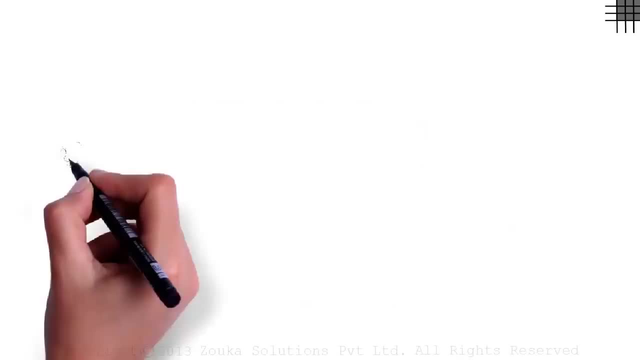 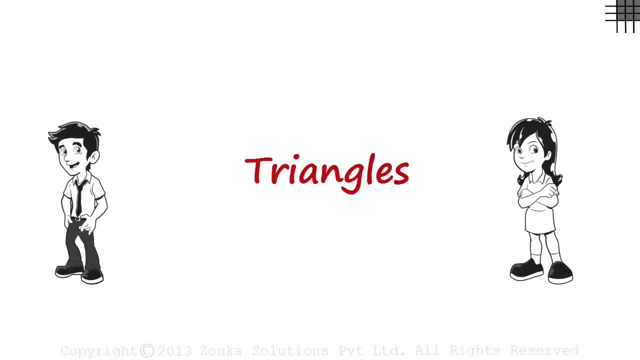 Let's play a very simple game. Zen and Zara will tell us how they've been working hard on constructing triangles. We just have to find out if they're telling the truth. First, let's hear Zen out. He tells us that he constructed a triangle. 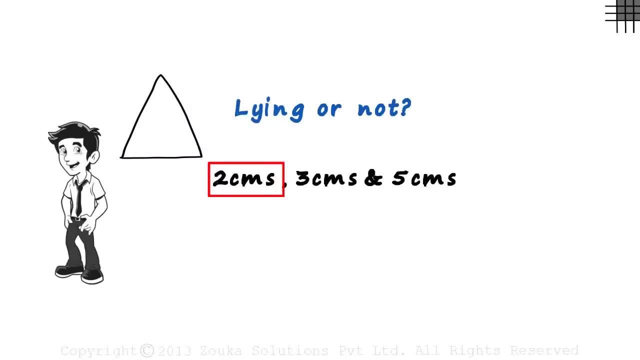 in which the lengths of the sides were 2 centimeters, 3 centimeters and 5 centimeters. Is Zen telling us the truth? Let's find out. We should use the triangle inequality theorem to find this out. The sum of any two sides should be greater than the third side. 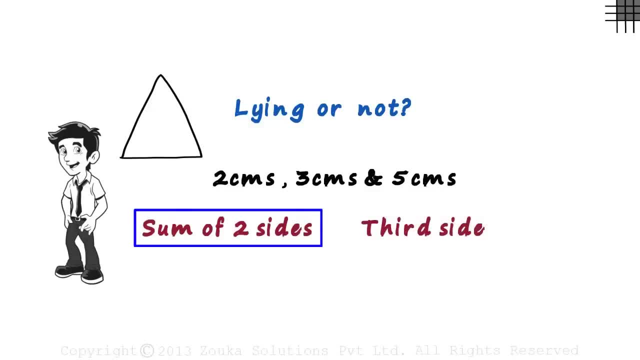 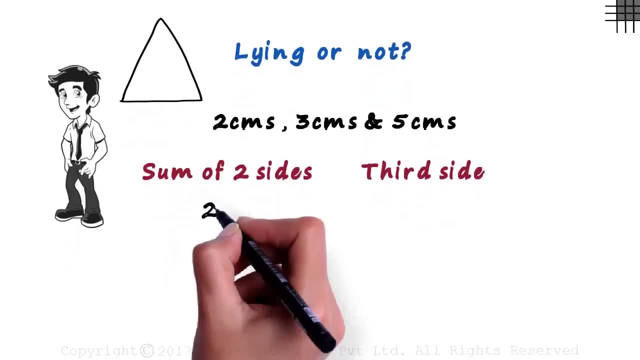 So we calculate the sum of any two sides and verify if it's greater than the third side. Let's find out the sum of the first two sides: It's 2 plus 3.. What is the third side? It is 5.. 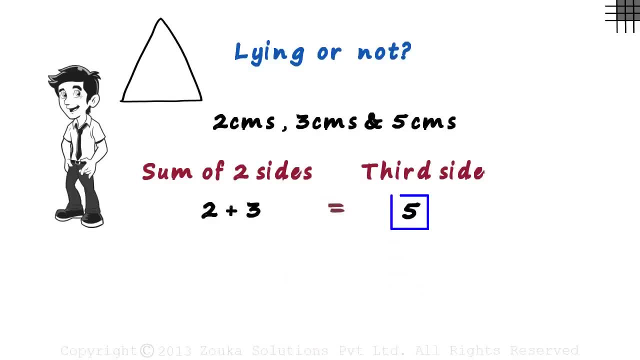 And we know that 2 plus 3 is equal to 5.. But the sum of two sides has to be greater than the third side. It means that a triangle with sides 2,, 3 and 5 centimeters cannot be formed. 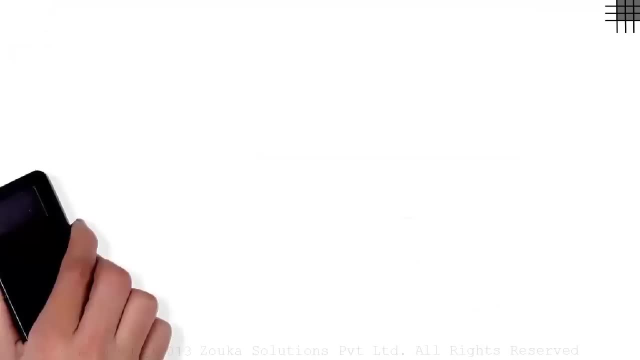 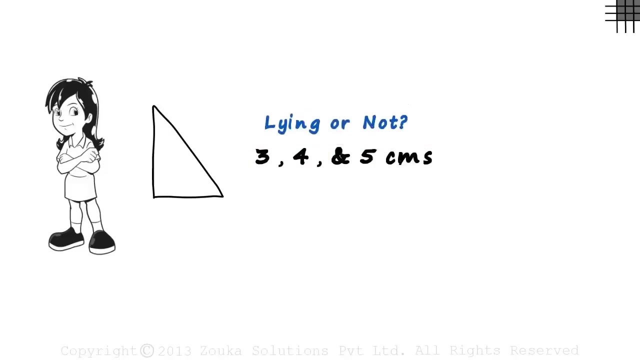 Zen was lying. Now Zara wants to tell us about the triangle she constructed. She tells us that the length of the sides of that triangle are 3,, 4 and 5 centimeters. Is Zara telling the truth? Let's make a small table to note the sum of two sides and the third side. 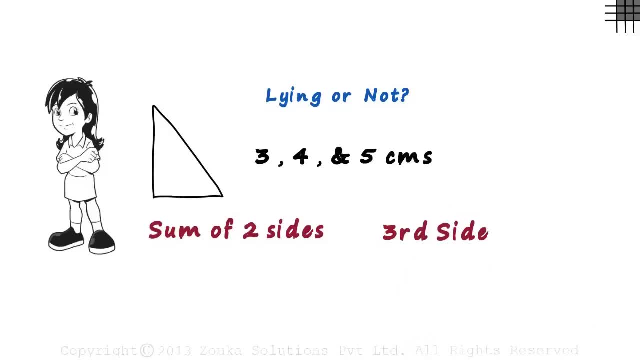 Remember, based on the theorem we learnt, the sum of any two sides should be greater than the third side. The sum of first two sides is 3 plus 4 and the third side is 5.. 3 plus 4 is greater than 5.. 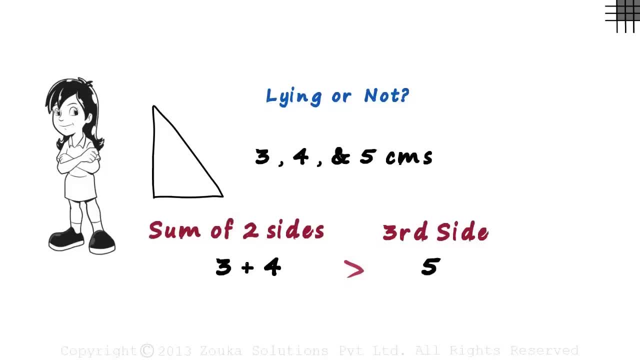 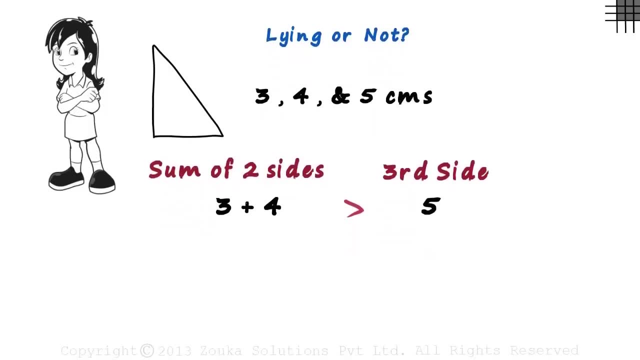 Can we conclude that Zara is telling us the truth? Not yet. We have just looked at one of the cases. Now let us consider the next combination: 4 plus 5.. The other side is 3. And the sum which equals 9 is greater than 3.. 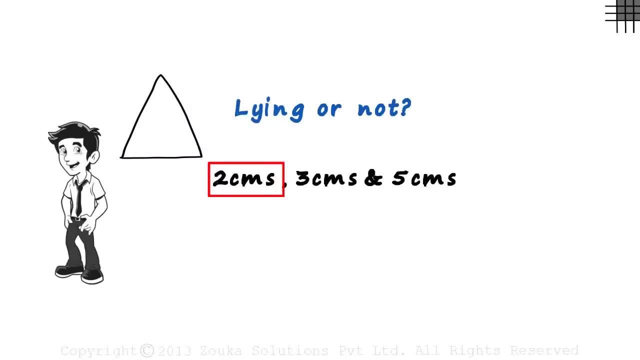 in which the lengths of the sides were 2 centimeters, 3 centimeters and 5 centimeters. Is Zen telling us the truth? Let's find out. We should use the triangle inequality theorem to find this out. The sum of any two sides should be greater than the third side. 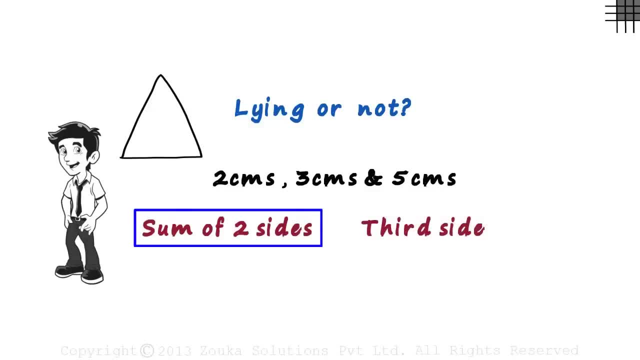 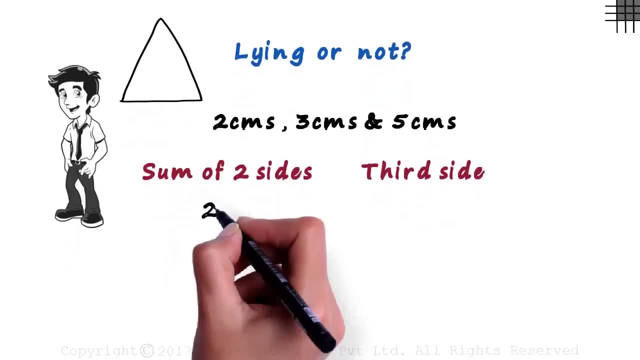 So we calculate the sum of any two sides and verify if it's greater than the third side. Let's find out the sum of the first two sides: It's 2 plus 3.. What is the third side? It is 5.. 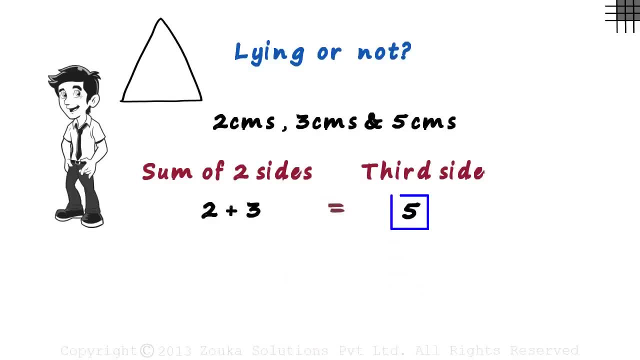 And we know that 2 plus 3 is equal to 5.. But the sum of two sides has to be greater than the third side. It means that a triangle with sides 2,, 3 and 5 centimeters cannot be formed. 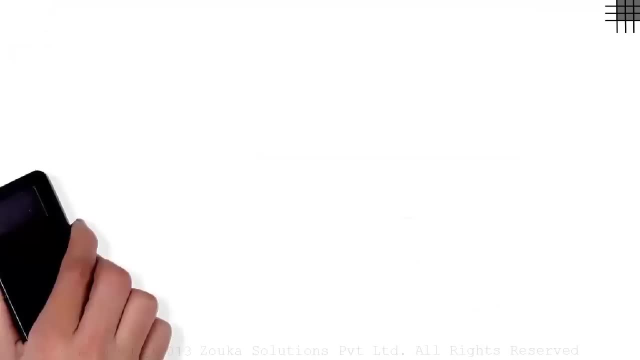 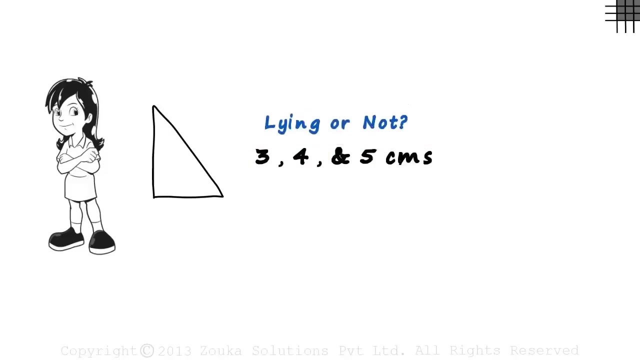 Zen was lying. Now Zara wants to tell us about the triangle she constructed. She tells us that the length of the sides of that triangle are 3,, 4 and 5 centimeters. Is Zara telling the truth? Let's make a small table to note the sum of two sides and the third side. 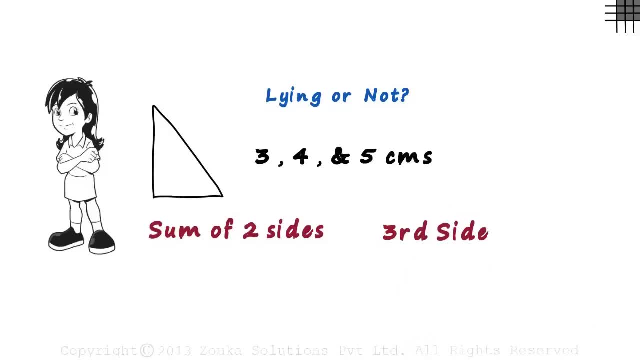 Remember, based on the theorem we learnt, the sum of any two sides should be greater than the third side. The sum of first two sides is 3 plus 4 and the third side is 5.. 3 plus 4 is greater than 5.. 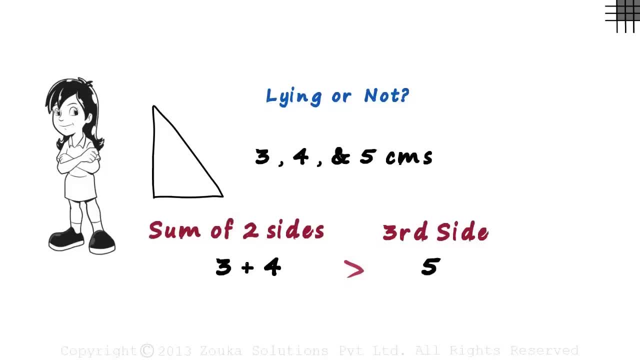 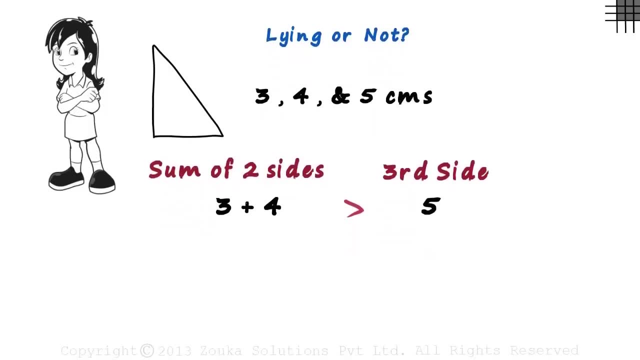 Can we conclude that Zara is telling us the truth? Not yet. We have just looked at one of the cases. Now let us consider the next combination: 4 plus 5.. The other side is 3. And the sum which equals 9 is greater than 3.. 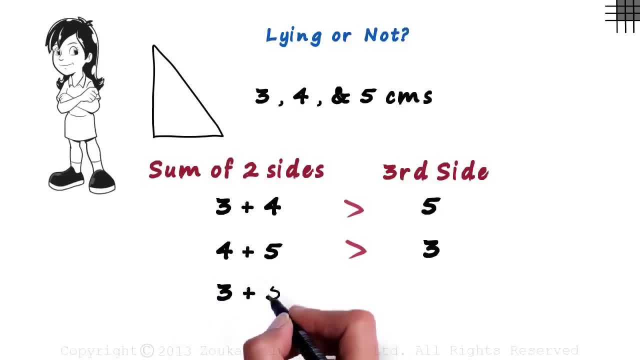 Now for the last combination, which is 3 plus 5.. The remaining side is 4, and 3 plus 5 is greater than 4.. So we can see that the condition is satisfied for all three cases. It means that a triangle with sides 3,, 4 and 5 centimeters can be formed. Zara was indeed telling us the truth.